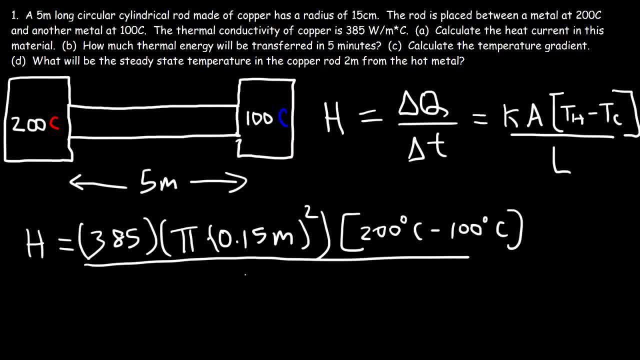 And then the difference in temperature. that's going to be 0.15 degrees Celsius, And then the length of the rod is 5 meters. So let's go ahead and type this in. So the heat current is 544.3 watts or joules per second. 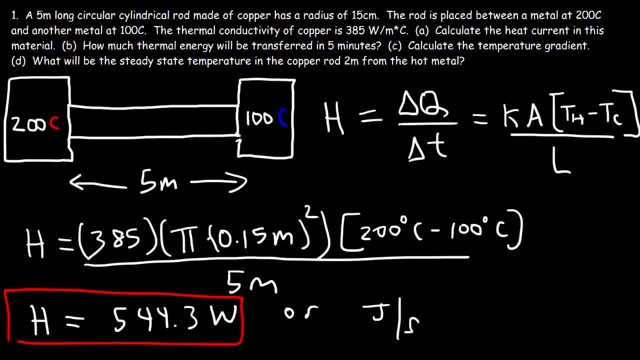 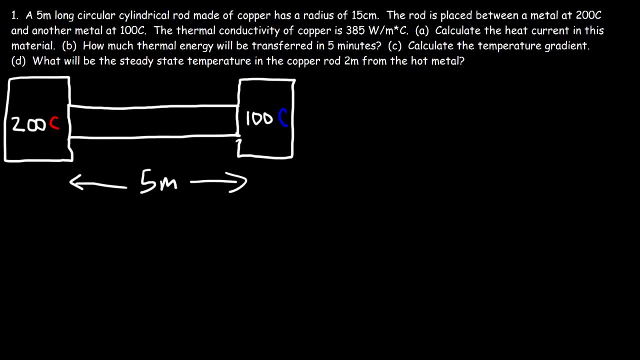 So the heat current is 544.3 watts or joules per second, And so this is the answer for part A. Now let's move on to part B. How much thermal energy will be transferred in 5 minutes? So we need to calculate Q. 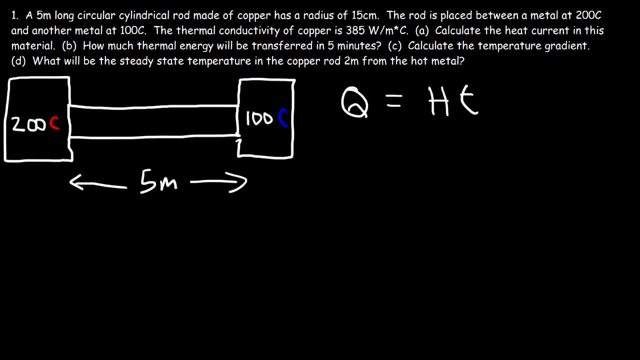 Q is going to be the heat current multiplied by the time, So we have the time in 5 minutes. We need to convert that to seconds, So there's 60 seconds in a single minute And we have the heat current in watts or joules per second. 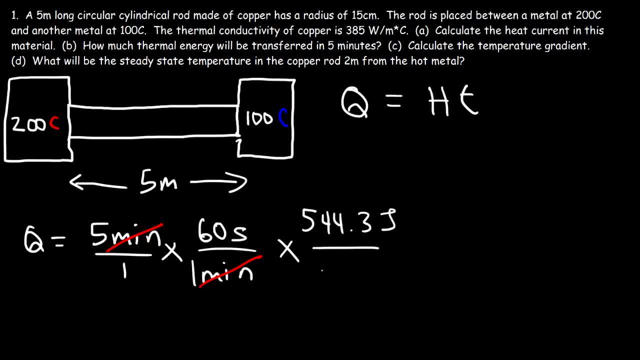 So 544.3 joules of thermal energy will be transferred every second, And so that's what the heat current tells us: how much heat energy is being transferred every second. And so 5 times 60,, that's the heat current. 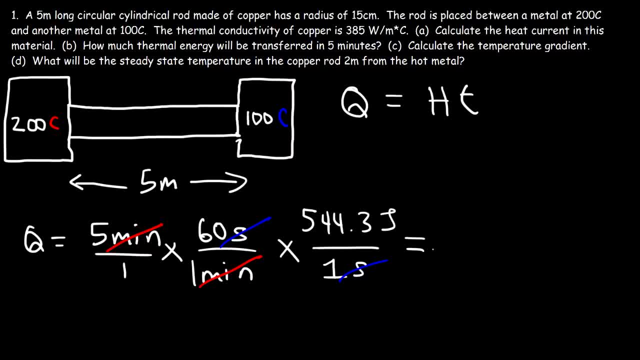 And so 5 times 60, that's the heat current. And so 5 times 60, that's the heat current- times 60 is 300 seconds. so 300 seconds times 544.3 will give us 163,290 Joules. 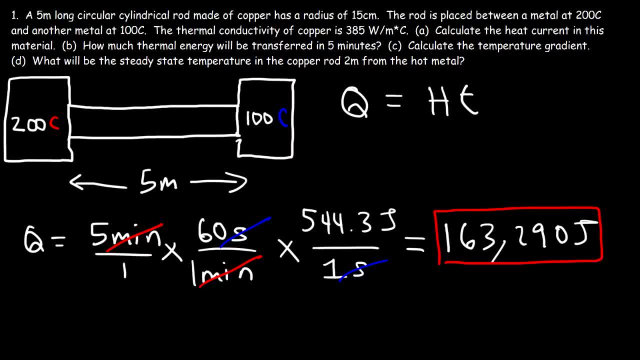 So that's how much thermal energy will be transferred in 5 minutes. So that is the answer to Part B. Now let's move on to Part C: Calculate the temperature gradient. So what is that? The temperature gradient is the change in temperature divided by the length. 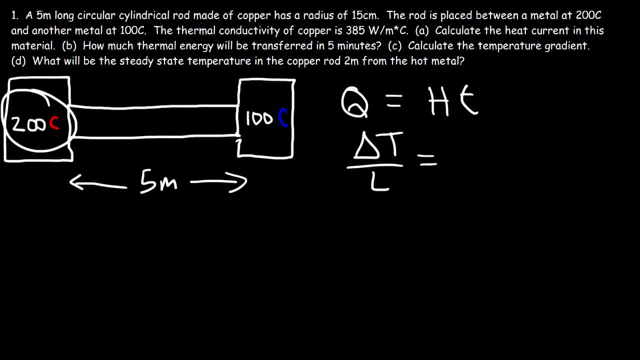 And in this example we have a difference of 100 degrees Celsius over a length of 5 meters. So the temperature gradient is 20 Celsius per meter. So that's the answer for Part C. Now Part D: What will be the steady state temperature? 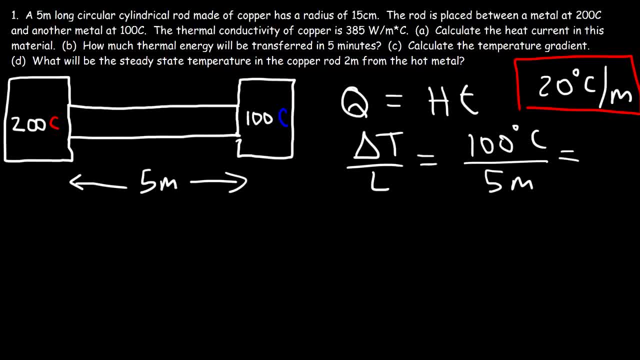 in the copper rod 2 meters from the hot metal. So I'm going to draw a bigger picture. So let's say this is 5 meters long And this is 200 and this is 100.. Now let's call this position 0.. 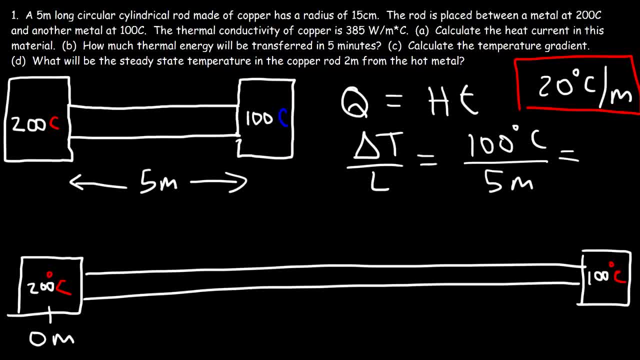 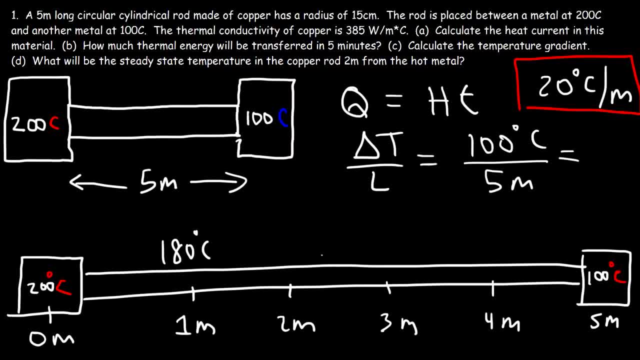 So 1 meter from the hot metal is going to be 20 degrees less, so it's going to be 180 degrees Celsius, And then another meter from that is going to be 160, and then 140, and then 120.. It's going to have basically 5 meters on the base. 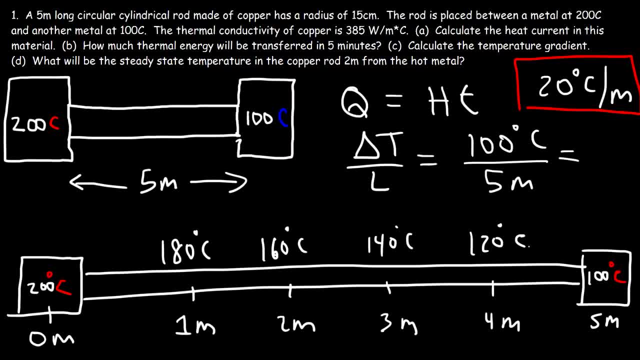 Good. So after some time has passed, if these temperatures are constant, if they remain at the values that they are, you're going to get a temperature gradient. Every meter, the temperature is going to drop by 20 degrees Celsius. So the answer to Part D: the final steady state temperature, 2 meters from the hot metal. 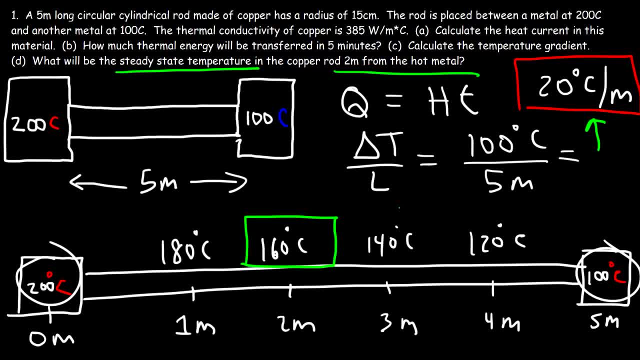 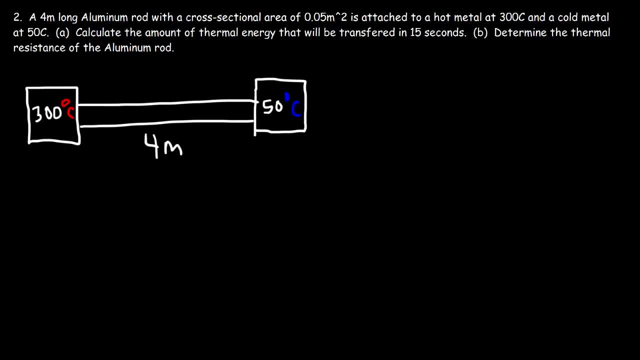 is going to be 160 degrees Celsius. So that's the answer. Number 2,: a 4 meter long aluminum rod with a cross sectional area of .05 square meters is attached to a hot metal at 300 Celsius and a cold metal at 50.. 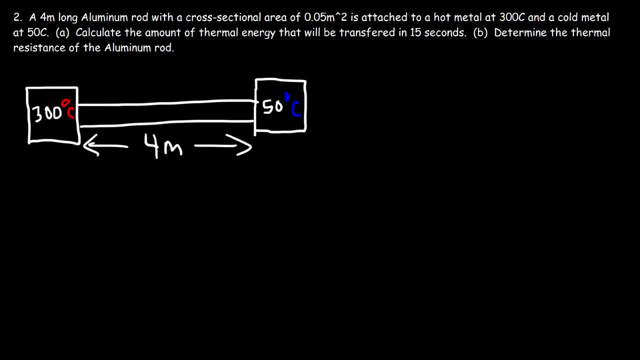 Calculate the amount of thermal energy that will be transferred in 15 seconds. So in this problem we need to calculate Q. So Q is going to be the thermal conductivity times the area Multiplied by the time in seconds, times the difference in the two temperatures divided. 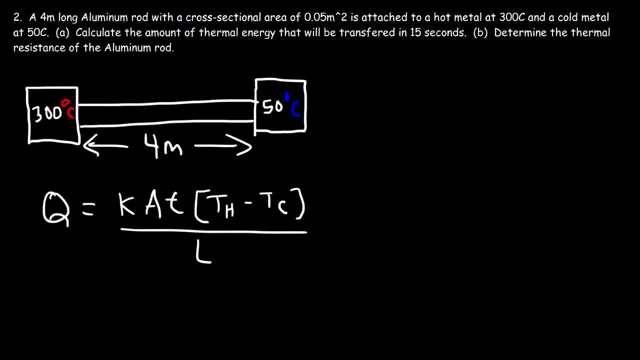 by the length. We're not looking for the heat current, which is the change in Q divided by the change in time. We simply need to calculate the total thermal energy that will be transferred. Now, the thermal conductivity of aluminum, which I'm going to give it to you now, is: 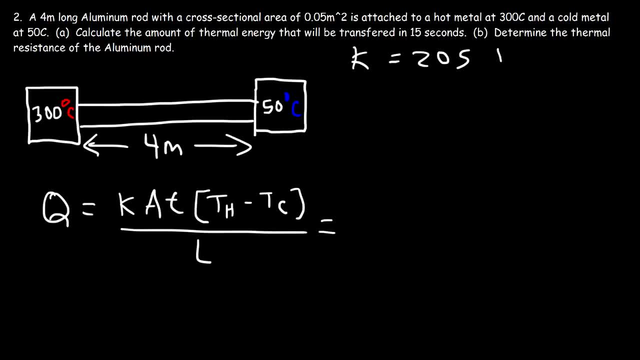 205.. And the units are watts per meter, And the units are watts per meter. And the units are watts per meter, And the units are watts per Celsius. So feel free to try this problem if you want to. The thermal conductivity K, as you mentioned before, is 205. 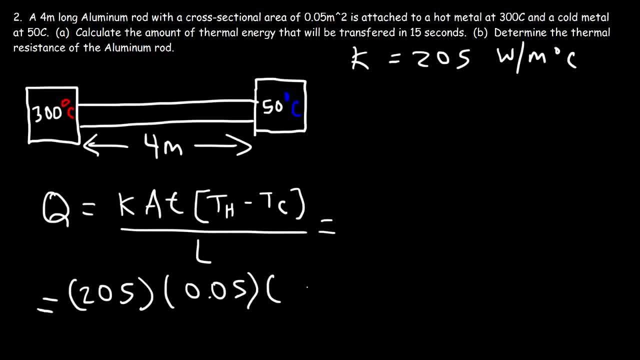 The cross sectional area is .05.. And the time is 15 seconds And the difference in temperature- 300 minus 50, is 250 Celsius And the length of the rod is 4 meters, So 205 times .05.. 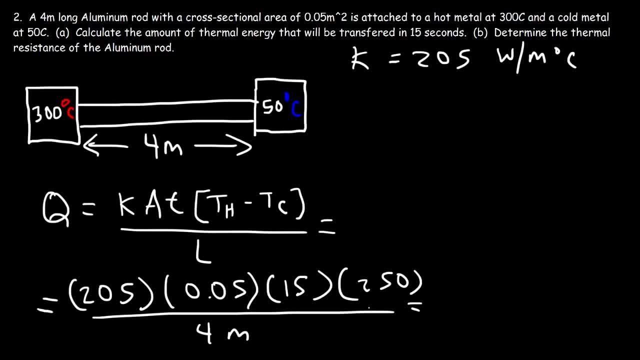 That's .05.. That's .05 times 15. times 250, divided by 4, is 9,609 joules. So that's the amount of thermal energy that's transferred in 15 seconds. Now, if you wish to calculate the heat current, it's simply delta Q over delta T, So it's 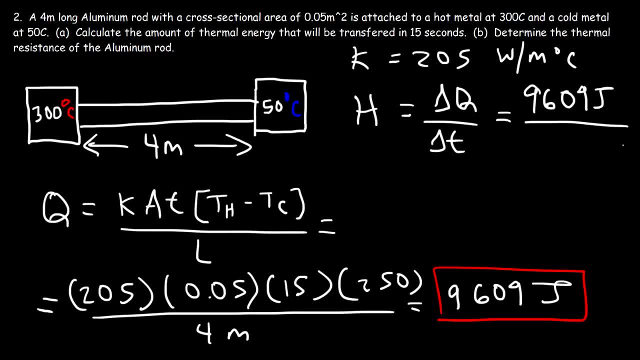 the amount of energy transferred divided by the time, which is 15 seconds, So you should get about 641 watts. So basically, the heat current is basically the power, the thermal power, which is work over time or energy over time. 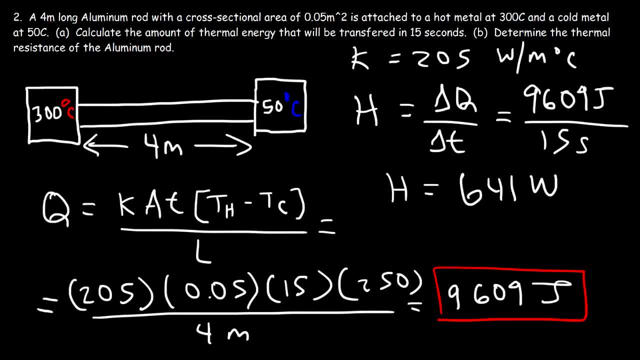 It has the same unit as power, which is watts or joules per second. Now let's calculate the thermal resistance of the proton, also known as antibiotic. The resistance of the proton is equal to the amount of energy transferred is over time. 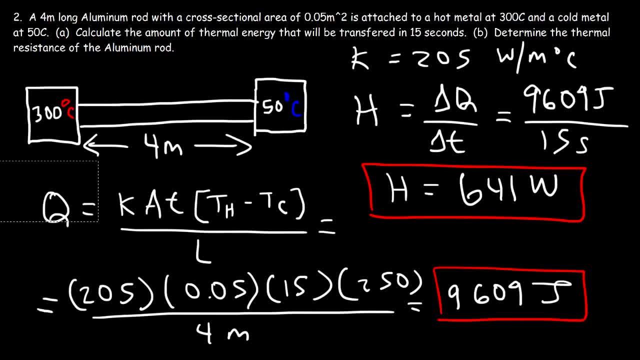 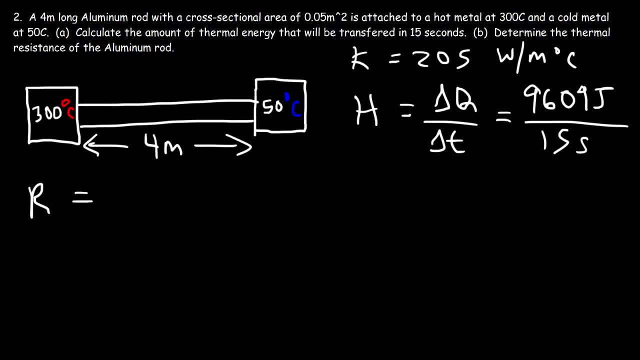 It has the same unit as the power, which is watts- Remember, Not Joules- rod. the thermal resistance is represented by the letter R and it's the left of the rod divided by the thermal conductivity. so we have a four meter long rod and the thermal conductivity is 205. so the thermal resistance for this 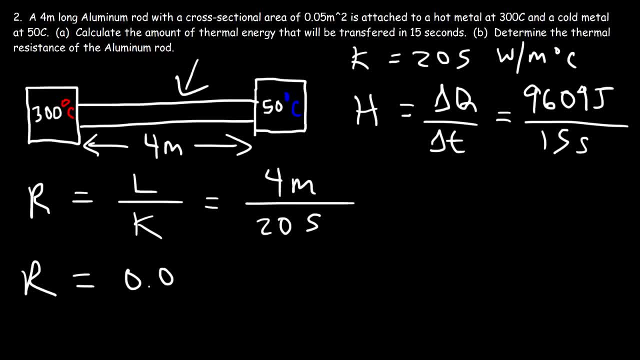 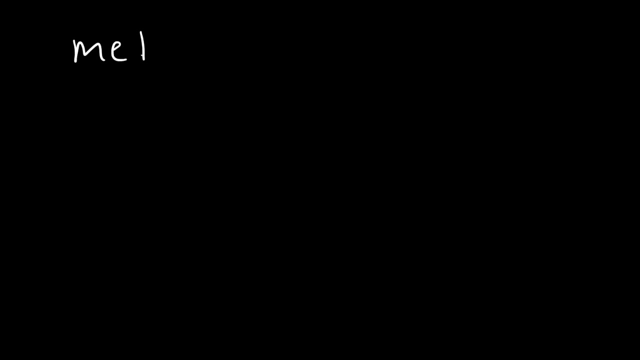 particular aluminum bar is going to be point zero one nine five, and the units are square meters times Celsius per watt. notice that the R value for aluminum is very low, and it makes sense because aluminum is a conductor. metals which conduct electricity very well have a very high K value but a low R value. so good conductors of heat like metals and 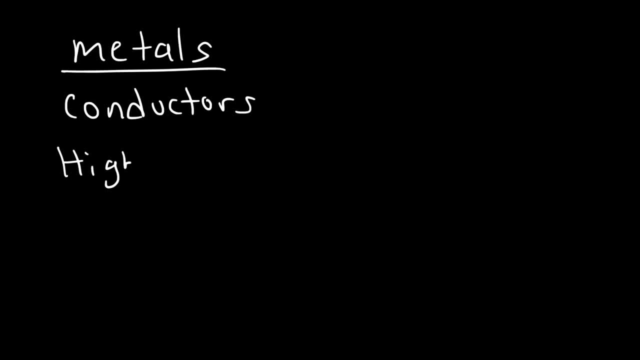 even diamond, they're going to have a high thermal conductivity value but a low thermal resistance. now, insulators like wood, fiberglass, air- if it's not moving, these will have a low thermal conductivity value because they don't conduct electric. I mean heat. very well, I was gonna say electricity but heat. but they will have. 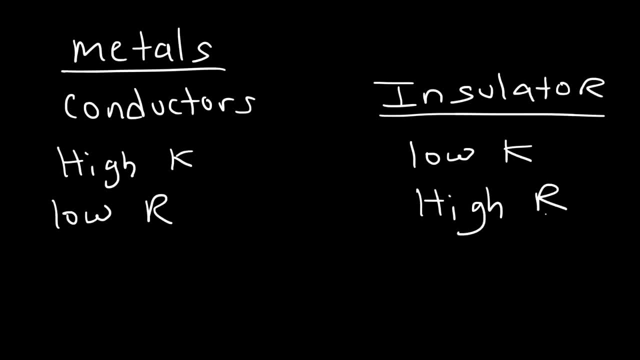 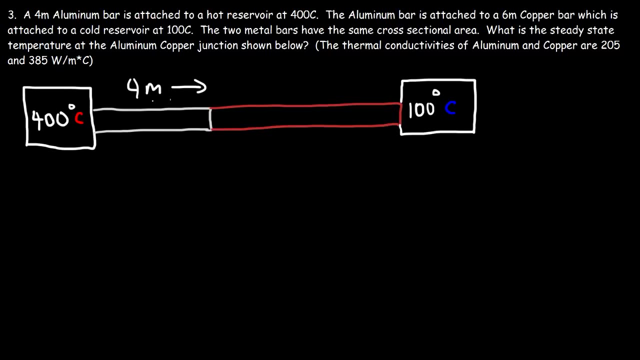 a high R value. so make sure you understand that insulators have a high thermal resistance and heat conductors have a high thermal conductivity. in this problem we have a four meter aluminum bar and it's attached to a hot reservoir at 400 degrees Celsius, and the aluminum bar is attached to a six and a half. 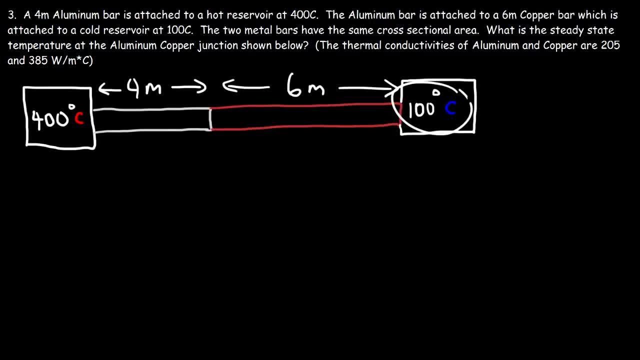 meter copper bar which is attached to a cold reservoir, and a hundred now. the two metal bars have the same cross sectional area and we have the thermal conductivity of each metal. what is the steady-state temperature at the aluminum copper junction shown below? so we want to find the temperature at that point. so how can we do this? what we 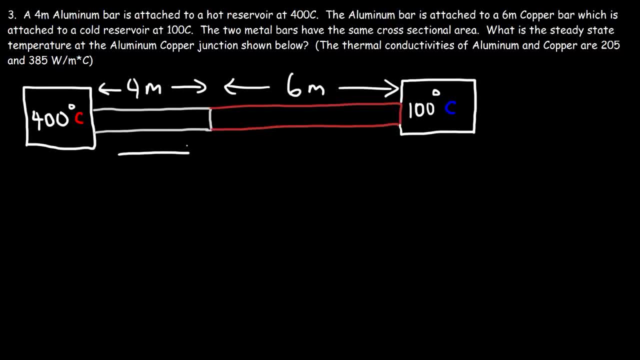 need to realize is that the heat current that flows in the aluminum bar is equal to the heat current that flows in the copper metal bar, and we know that the heat current is equal to the thermal conductivity times the area times the temperature difference divided by the length. so what we're going to do is set. 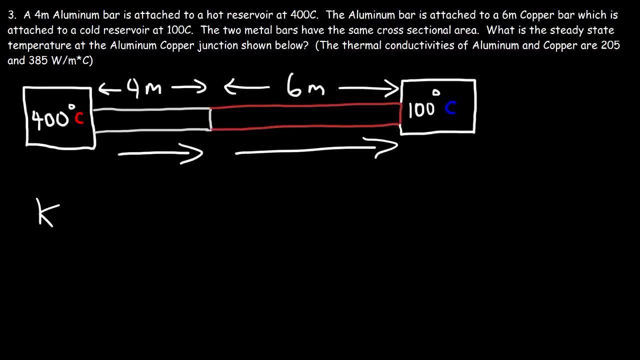 the heat current in the aluminum bar equal to the heat current in the copper bar. so this is going to be K for the aluminum bar times, the area times the temperature of the aluminum bar at the hot reservoir. now the cold temperature for aluminum is basically this temperature, so I'm going to call that T. 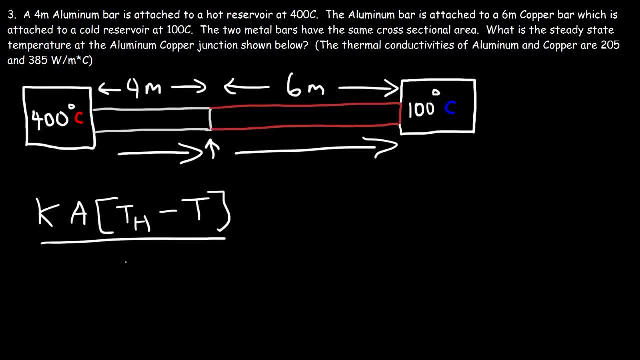 that's the T that we're looking for, divided by the length of the aluminum bar, and then for the right side, is going to be the thermal conductivity of copper times, the cross-sectional area. now, this part is the hot temperature for copper, so I'm going to call that T and the cold. 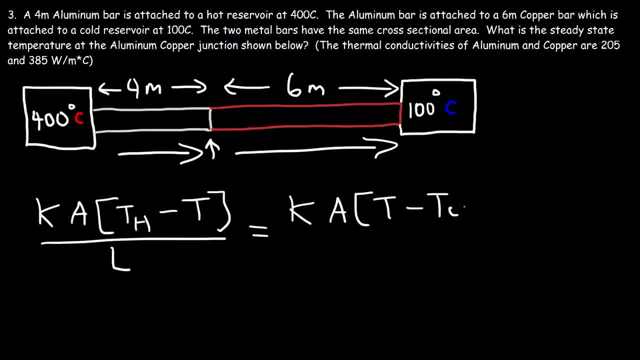 temperature for copper is TC, or, which is a hundred divided by the length of the copper bar. so make sure you understand. the left side is for aluminum, the right side is for copper. now let's go ahead and plug in the values. now both metal bars have the same cross-sectional area, so we can cancel A the thermal. 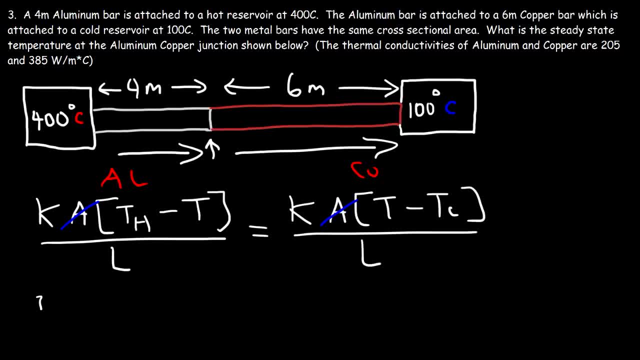 conductivity for aluminum is 205 and the hot temperature reservoir for the aluminum metal is 400. the length of the aluminum bar is 4 meters and for the copper bar is 6 meters. the thermal conductivity of copper is 385 and the cold temperature reservoir is 100. so now we just got to do math and 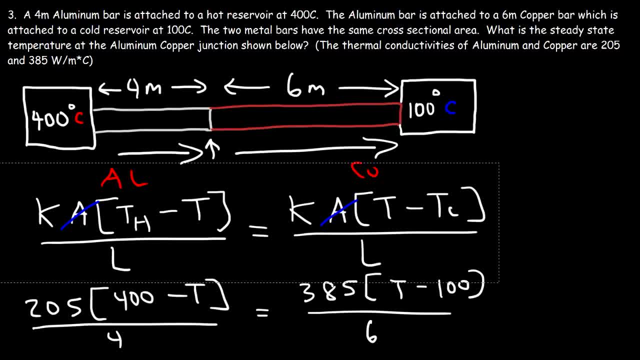 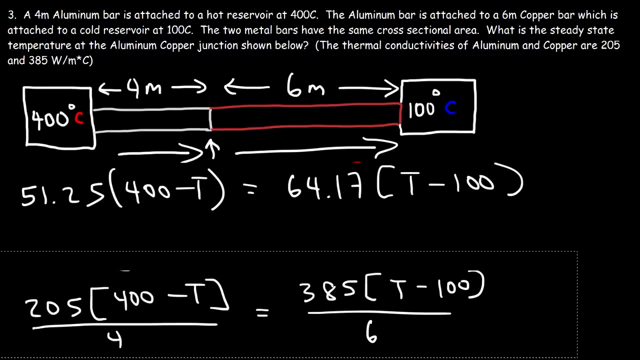 solve for T: 205 divided by 4 is 51.25, and 385 divided by 6, that's 64.25. point 17. now on the left side, let's distribute 51.25 to 440 minus T, so 51.25 times 400. 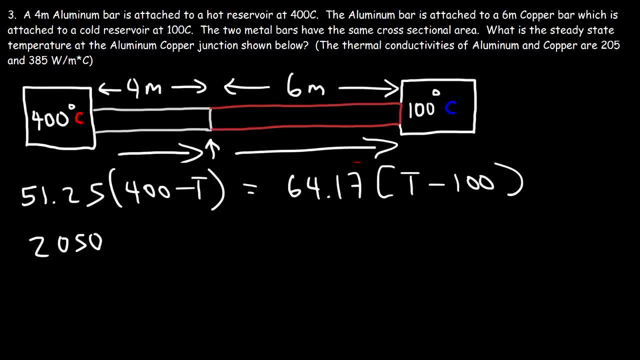 that's 20,500 and then minus 51.25 T. on the right side we have 64.7 T minus 64.7. On the right side we're going to have 64.17 T minus 64.17 T minus 64.7 T minus 64.7. We have 64.17 T minus 64.7 t and the cold temperature reservoir at the end of here is a 64.2.. And now, if we look at this part, we'll be able to use the formula to solve for T a hundred times, 3.5 times. the hot. cold temperature reservoir for copper is 60.4 and the hot temperature reservoir is 4.6.. 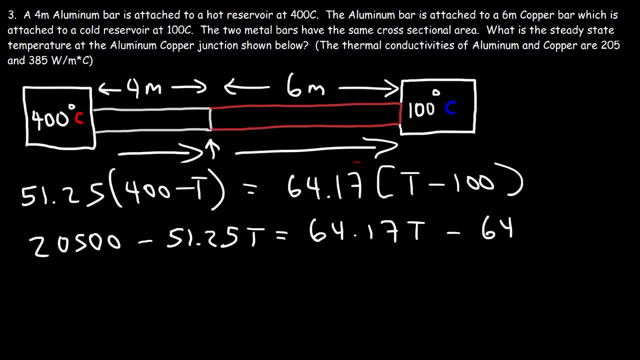 times 100 is 64: 17. so now let's add a 51 point 25 T to both sides and let's add 64: 17 to both sides. so twenty thousand five hundred plus 64: 17, that's twenty six thousand nine seventeen, and on the right side we got sixty four point. 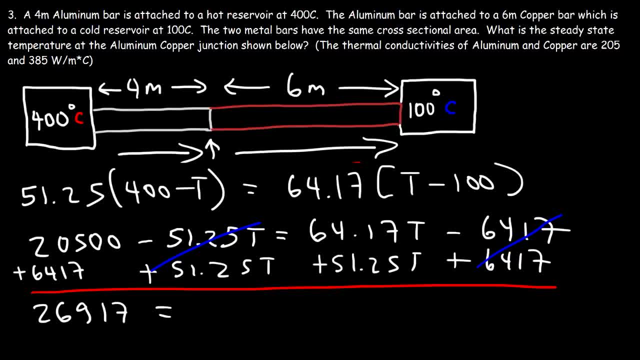 seventeen plus fifty one point twenty five, and so that's a one fifteen point forty two. so twenty six thousand nine seventeen divided by one fifteen point forty two, that will give us a temperature of 233 Celsius, which is in between 400 and 100. so that answer makes sense. 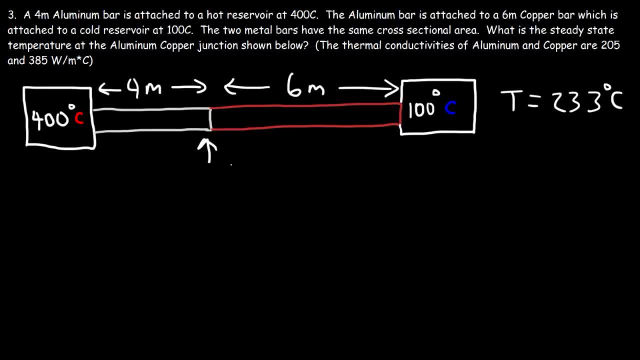 so at this point, the temperature is this value. now let's calculate the temperature gradient in the aluminum part and the copper metal. so right now, for this problem, this is the final answer. but we're just taking this problem and that step further. so keep in mind: the temperature gradient is the change in temperature divided by 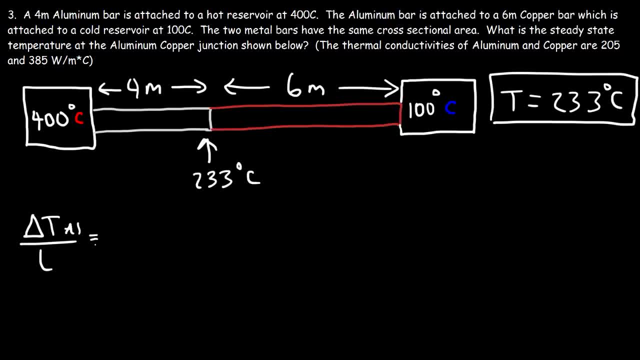 the length. so in a case for the aluminum Bart, the temperature differences for 100 minus 233 divided by 114, so it changes 41.75 degrees Celsius per meter. now the temperature gradient and the copper bar is going to be 233 minus 100, so that's. 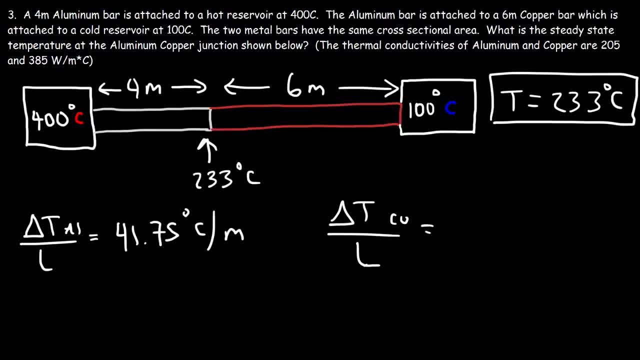 the temperature difference of 133 Celsius divided by 6 meters. so the temperature gradient is 22.167 Celsius per meter. so now we can calculate the temperature along these two rods at every meter. so let's say this is 0. so at 1 meter the temperature is going to be 400 minus 41.75. so at this point it's 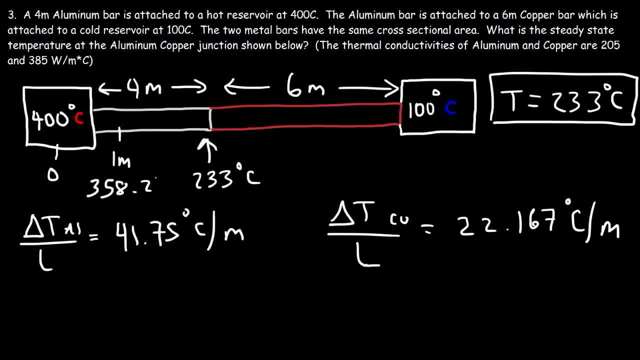 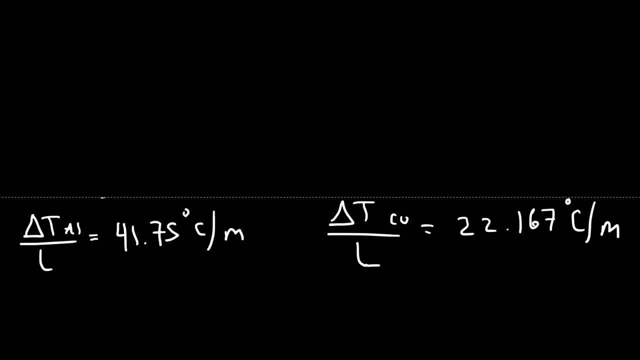 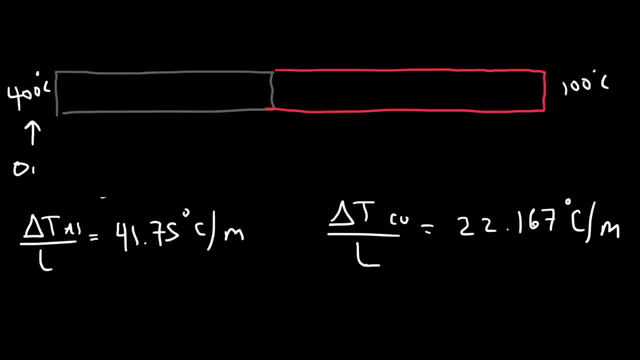 hundred and let's call this 0. so at 1 meter, we said the temperature is going to be 358.25. now, at 2 meters, it's going to be 358.25 minus 41.75, so the temperature is going to be 316.5 Celsius. 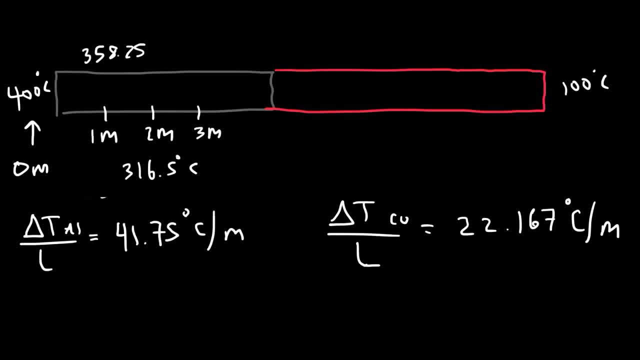 and at 3 meters it's 316.5 minus 41.75, so it's going to be 274.75, and at 4 meters, if you take 274.75 minus 41.75, you get 233 Celsius. now at 5 meters we 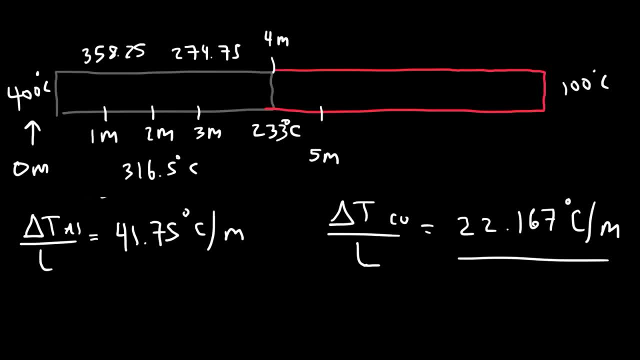 need to use the temperature gradient for copper now. so it's 233 minus 22.167, and so the temperature is going to be 210.8 degrees Celsius, and then at 6 meters, and It's 210.8 minus 21.167, so it's going to be about 189.6.. 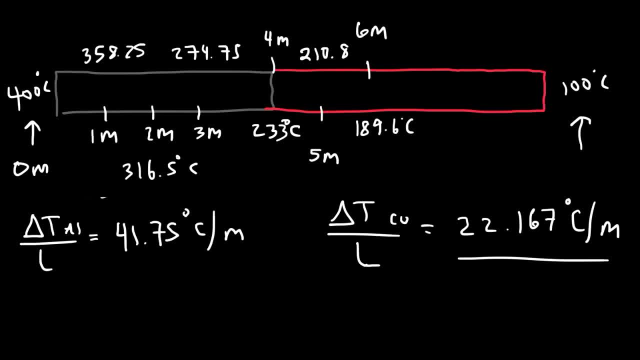 And you can keep doing this until you get to 100. So the temperature gradient tells you the temperature change along the rod every meter. So that's it for this video. Hopefully this gave you a good understanding of heat currents. thermal conductivity, thermal. 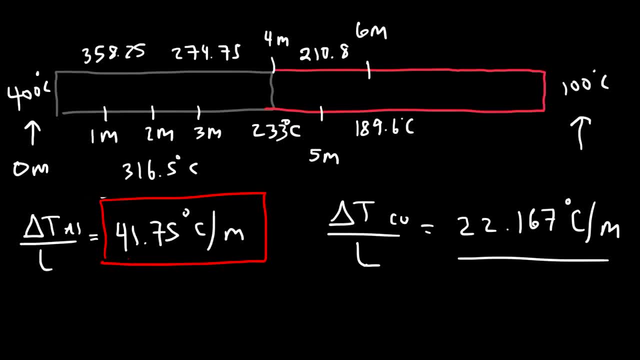 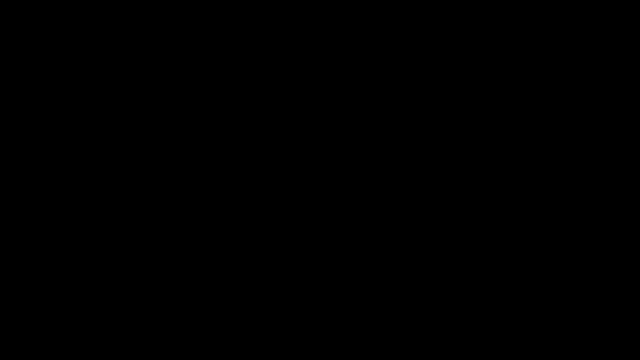 resistance and temperature gradients along the metal. Thanks for watching Subtitles by the Amaraorg community.